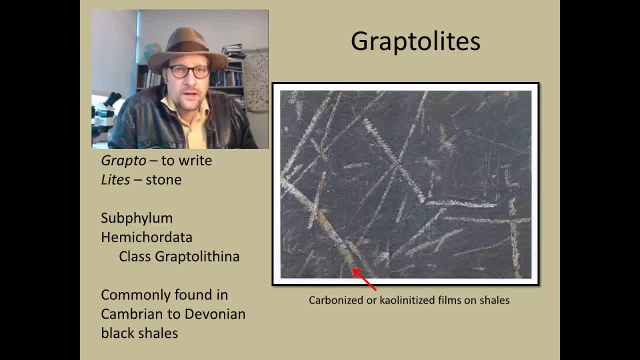 So graptolites are actually what they are: carbonized or kaolinized films that are on the shells. So this is sort of the remnants of the organic matter that compose their bodies that are preserved in the rock record. So they don't have calcium carbonate and hence they're not big reef builders. and 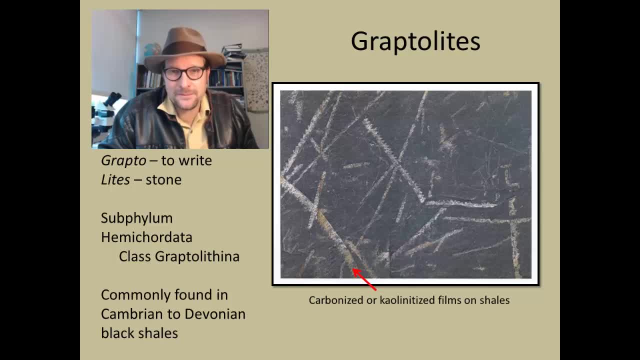 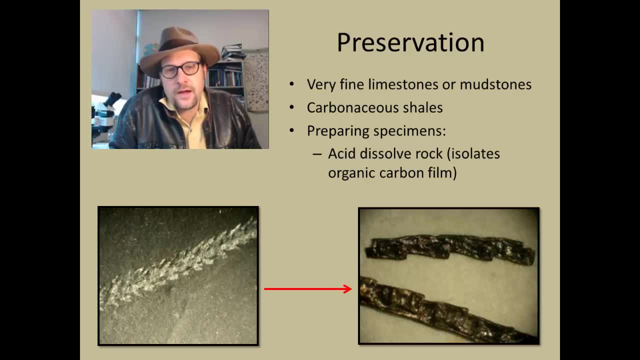 they're sort of peculiar. We'll talk a little bit about what these things might actually be. So the preservation is very different, in terms of graptolites, than the other fossils that we have seen so far in this class. They're found only in very fine limestones or mudstones or carbonaceous shales. 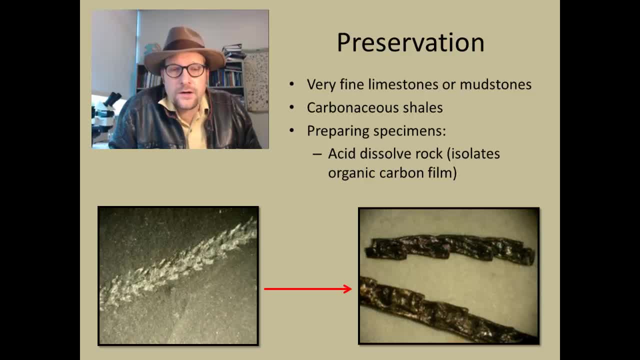 When found. they look like little marks on the shale and these are sort of remnants of the original organic carbon that's been carbonized or turned into coal or something like that. In preparing the specimens, what scientists have done and paleontologists have done that, 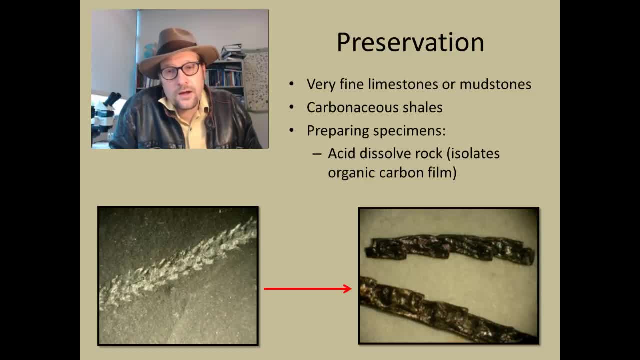 study graptolites is that they dissolve the rock, usually in a combination of hydrochloric acid. They'll get rid of the calcite cement and then they will use hydrochloric acid, which will get rid of some of the silica. 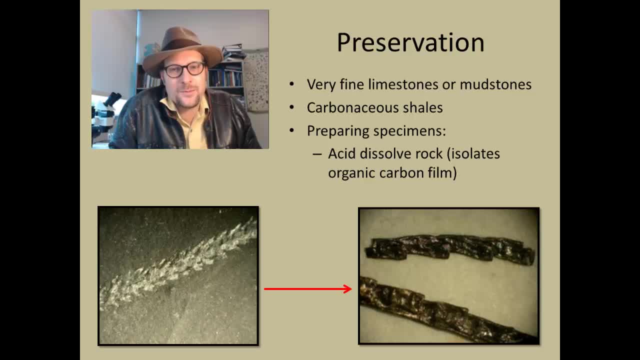 And that leaves behind a sort of the organic carbon film, the original fossil. It's a very delicate process and only a handful of specimens have been prepared this way to such detail that we can kind of study these things in three dimensions. Most graptolites are found in two dimensions, sort of squished between the layers of shale. 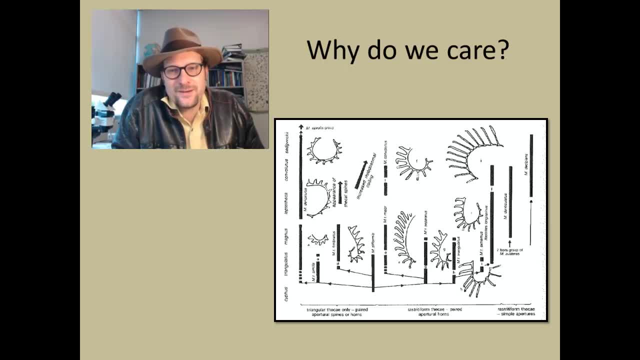 So why do we care about graptolites? What's their meaning? What's their purpose? in geology, Graptolites are a very interesting group in the fact that they are readily preserved and they can be identified to different species. Now, these species are a little bit different than the species we've been talking about. 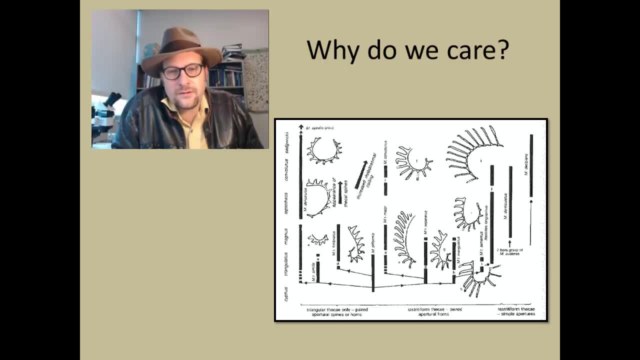 in that we don't have preserved the entire body. Oftentimes, it's these little graphs, these little fragments of these fossils that are preserved, And they're often preserved in these black shales, Where we may not have any other fossils to go on. 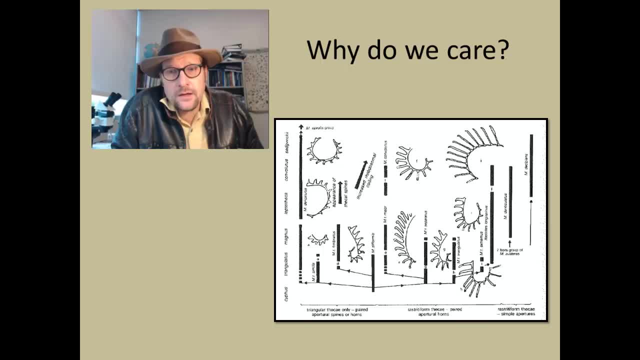 So graptolites came to importance in biostratigraphy in being able to map out different biozones in the rock record, in particular sedimentary rocks where you don't typically find many fossils in. Let's talk about the first order, the order Graptoloididae. 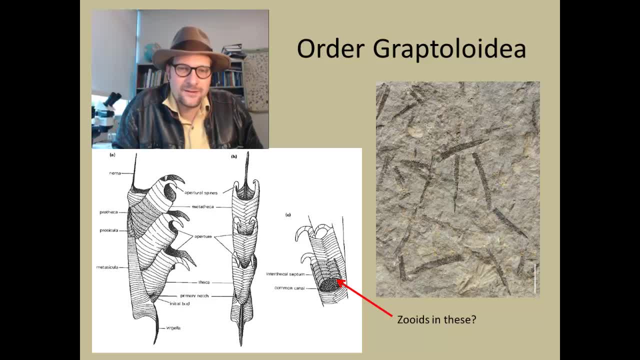 This is a group in which we've prepared out some of the specimens to get kind of a look at sort of the anatomy of what these things are. So they oftentimes will have little spines that go up and down them, so they kind of 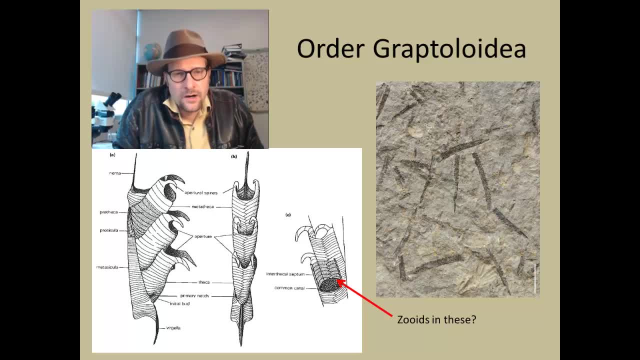 look like razor saws, And what those are are basically surrounding these little openings, these little apertures, which possibly housed a zooid. So these are probably colonial organisms, though it's difficult to say that a zooid of some sort would live in. 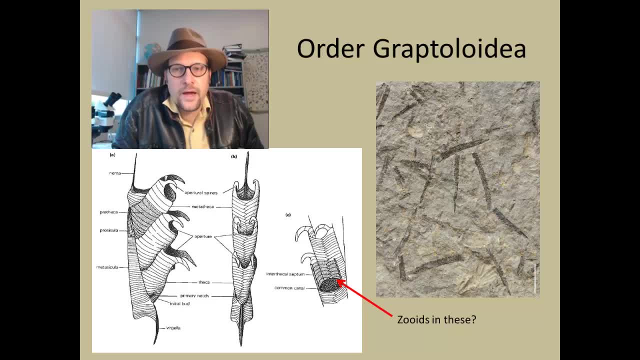 And then each one of these little openings, Each one of these little openings is a zooid. Each one of these little openings is a zooid. Each one of these little openings, these little apertures along these sort of razor blade edges of these things, was home to sort of colonial organisms. 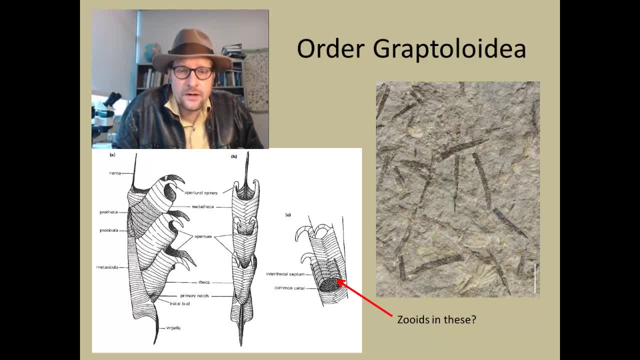 What's interesting about these colonial organisms is that they are interconnected, And so many scientists have hypothesized that a nerve cell ran between the zooids that allowed them to sort of communicate with each other, And as such, they're sort of in between a colonial organism and a single organism. 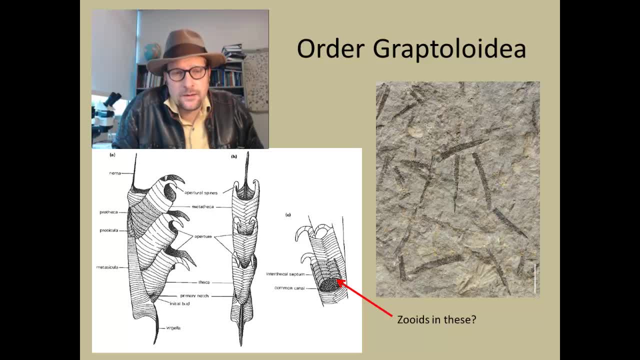 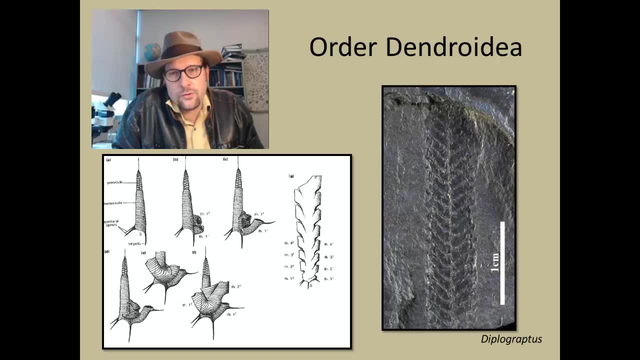 They're very peculiar And the way that they form their skeleton. The other order is the order Dendrodoidae. The other order is the order Dendrodoidae. These tend to be ones that seem to be more attached. It's hypothesized that these guys may have been more sessile, although there are some. 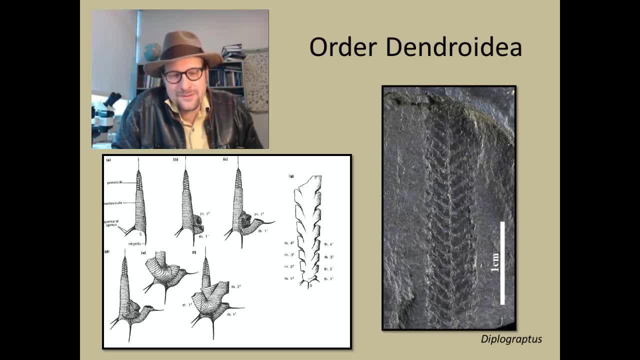 that are probably floaters, So these might have been sort of like growing. So these might have been sort of like growing Like a plant. Again, they have openings, apertures that grow out, composed of this organic matter that they compose their skeletons. 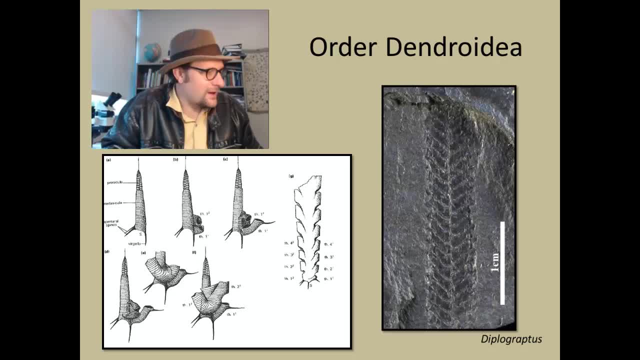 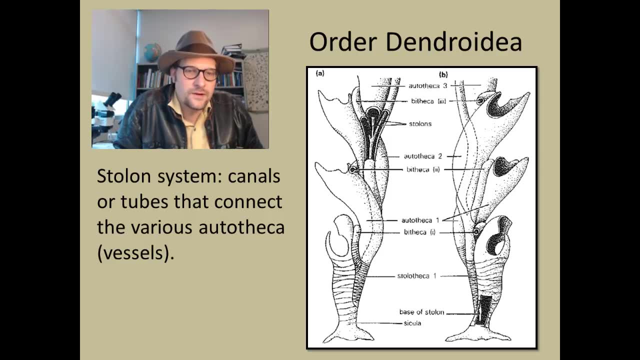 A good example is Diplographis here, an example of one of those Dendrodoidae, The order Dendrodoidae, have these Stolial systems, these canals or tubes that connect the various autothecia, these little vessels. 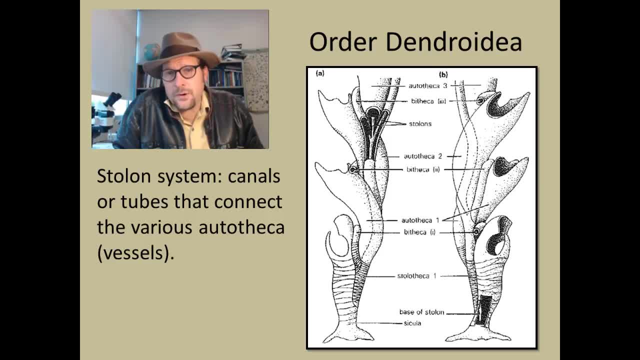 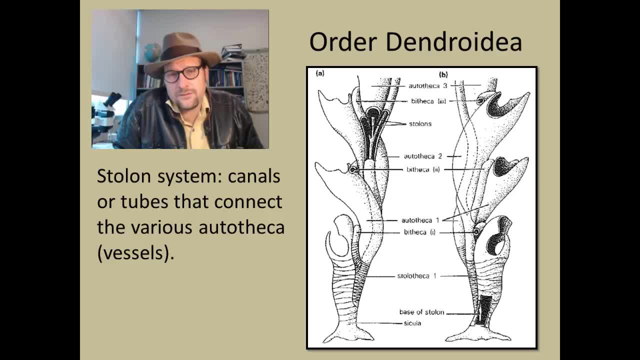 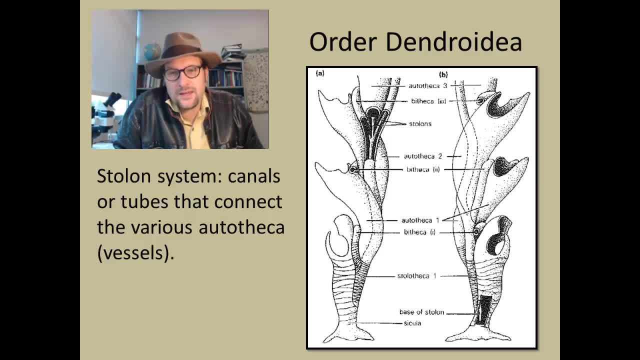 So one of the main reasons that these skeletons were pronounced and form quite a bit of the skeleton of these things, it's made out of organic carbon connecting each of these apertures that house some sort of creature, some zooid that probably was filter feeding. 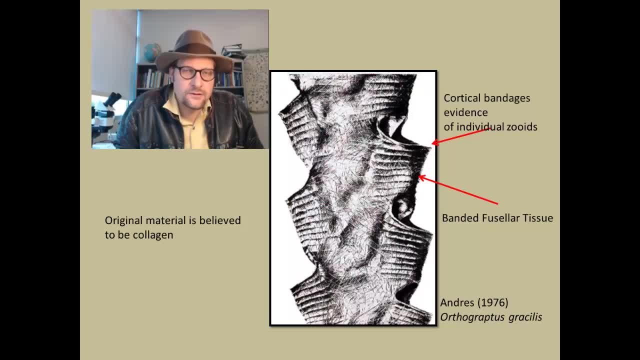 Now the skeleton itself is made out of collagen, or that's at least what scientists believe the original matter was composed of, And, of course, when it's buried under heat and pressure- and these are very old Devonian to Cambrian- that the original collagen breaks down into smaller units of carbon and hydrogen bonds. 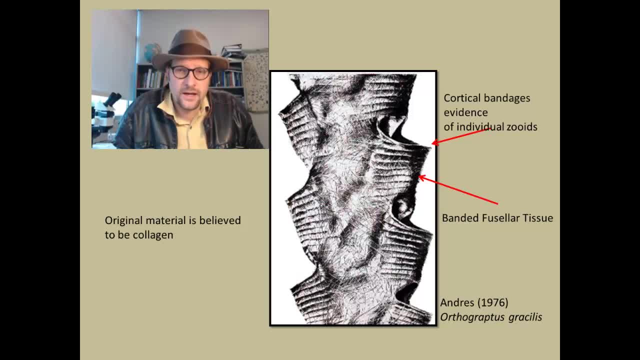 but probably was originally collagen, some sort of organic matter that held these things together. One of the things that's really interesting is you get these coracle bandages and these are evidence that in each one of these little cups there was an individual zooid and they 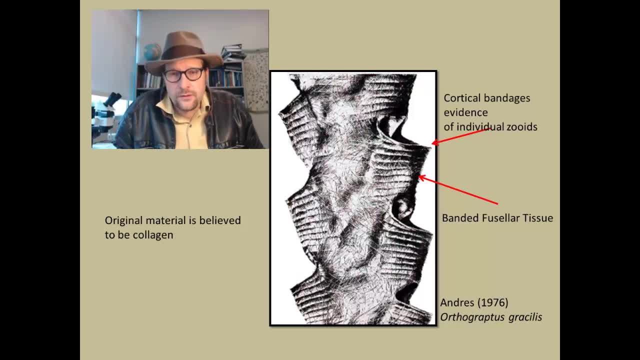 communicated with each other through a stoma system. You see banding on the edge underneath the apertures and this is usually interpreted as growth rings of the zooid. So the zooid would basically build up those growth rings around the aperture as it grew over time. So this is 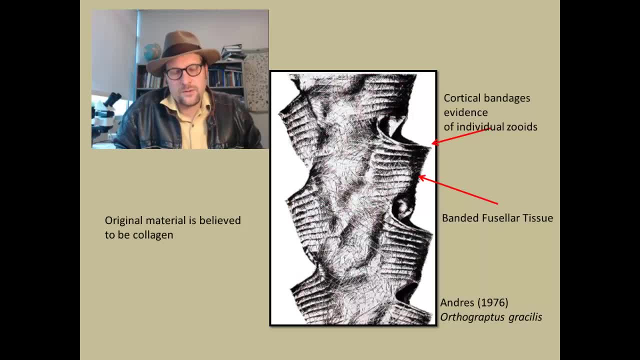 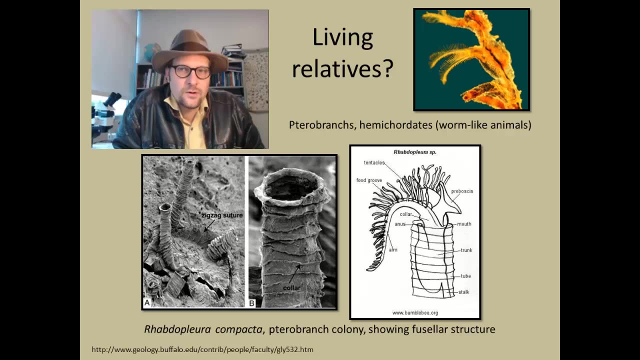 an example of a very nice, probably one of the best examples of a three-dimensional image of a graptolite in detail. This is Orthographis gracilis. Now, one of the interesting things about graptolites is that we're starting to kind of get a clue of what they might actually. 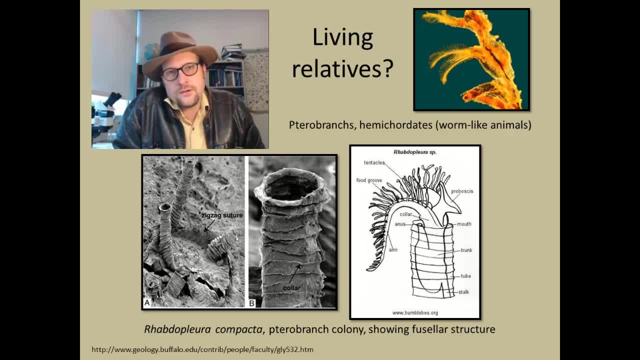 represent and some possible living relatives that do this type of skeletal growth using collagen. They appear to be closely related to the petrobranks. These are the members of the hemichordates, a worm-like creature. They are also known as the petrobranks. 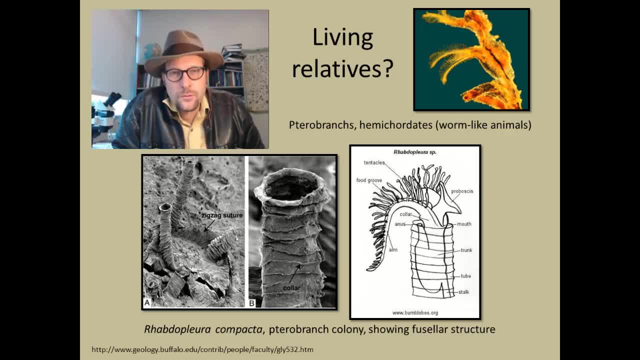 These are creatures that live in the ocean. These include the tubeworms that you often see in deep sea vents that were discovered in the 1970s when oceanographers went into the deep sea vents. They build their tubes out of collagen that they grow, And here's an example of 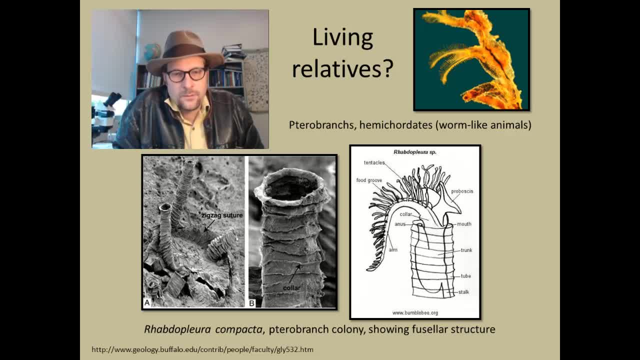 Raptoplura compactia. This is a pterobrachian colony and they basically are these little things that have a, they have sort of a food tentacles that come out. They have a proboscis, They wave those tentacles back and forth and are filter feeding In the deep sea vents. they 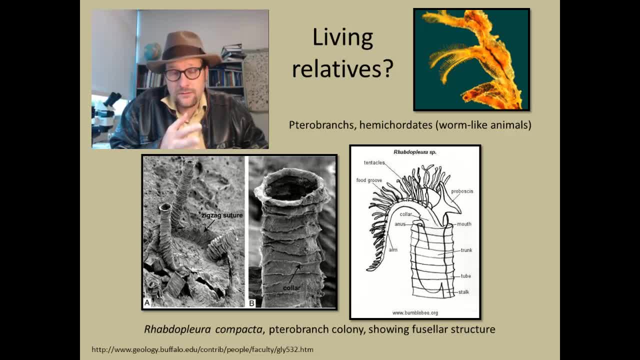 actually can do some exchange with some of the bacteria that feed on the hydrogen sulfide in deep sea vents where there's no sunlight getting down there, And then they basically secrete around their structure this skeleton, this tube that holds them in. It's made out of collagen and you 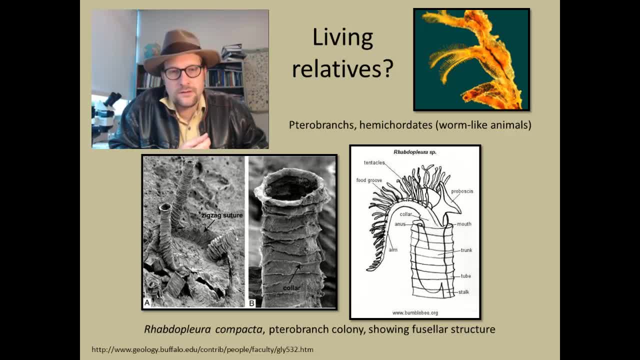 have some of the similar structures that we see in the graptolites in the fossil record, where they basically secrete this collagen around to form these like tubes that they can live in And then they can retract into these tubes. So it's not calcium carbonate like we saw with the bryozoans. 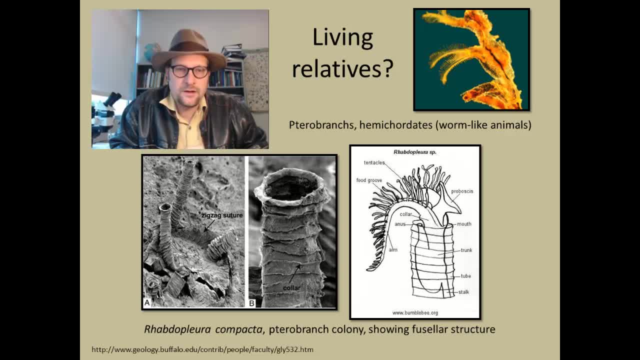 or brachiopods. This is collagen that they're basically exuding, And then they have this portion that comes out and does the filter feeding with tentacles that comes out- The term itself. Now, living petrobranks have a fossil record that actually extends all the way back to 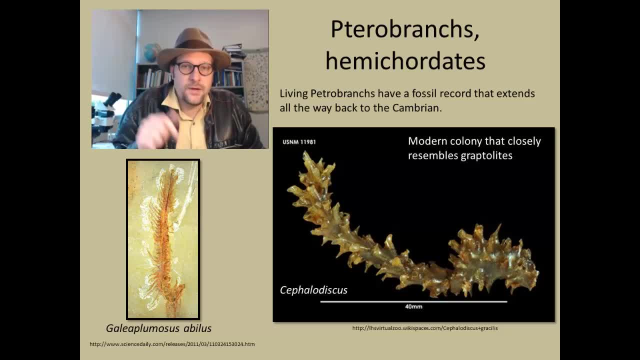 the Cambrian- Here's an example of one of the Cambrian petrobranks- has a fossil record And the modern cephalodissaculus here. in fact, if you look at it, it's skeleton- that the colony of skeletons made a collagen of a modern one. This is one now, the Smithsonian Museum. 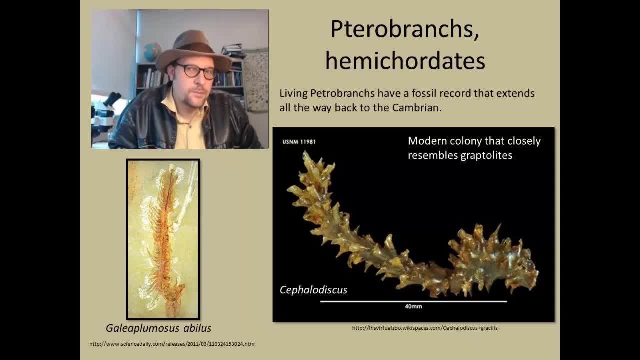 You'll note that it has a very similar type of structure that we see in the graptolites, And so it's thought that the graptolites were sort of an early branch off the hemichordates and survived in a little bit. 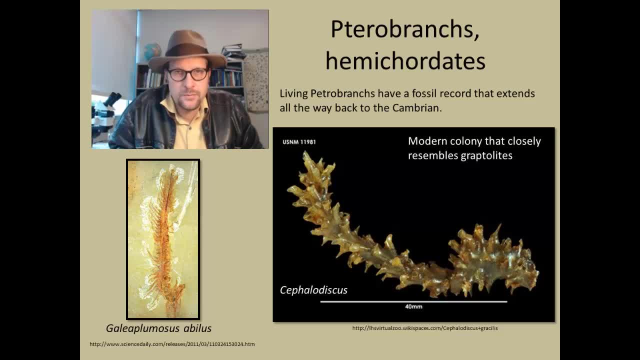 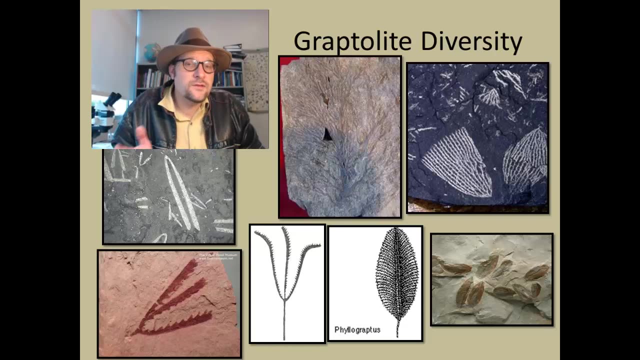 different ways than modern petrobranks that live kind of deep in the ocean And what they did was basically be floaters, be planktonic, rather than necessarily being tied down or being sessile, Although some of the graptolites were sessile organisms. Now graptolites are really diverse. 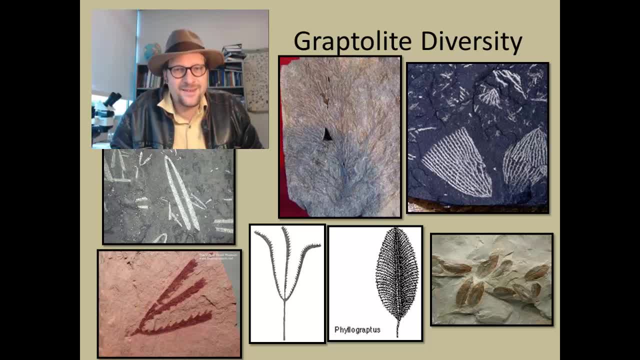 I mean there's all sorts of shapes and sizes of graptolites that are found in the rock record. Many, many different types of graptolites have been described, And they can be easily identified too, just by having a splitting. 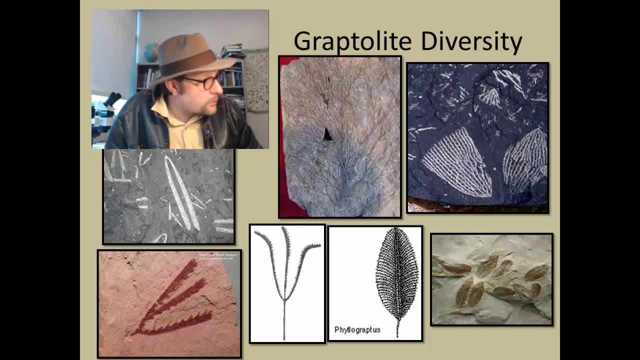 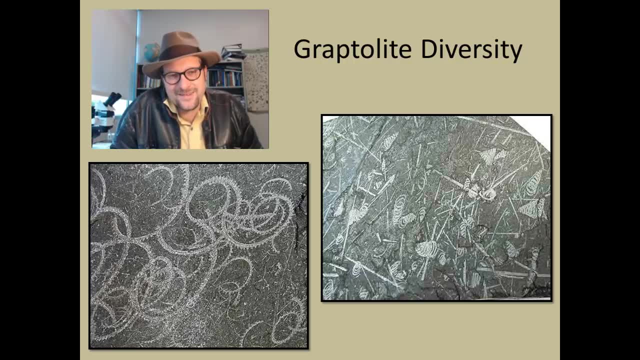 a shell and finding some of these really interesting things, An incredible amount of diversity of graptolites. Some of the weirdest graptolites are these. These are just bizarre. They almost look like gears or they don't really look like organic. 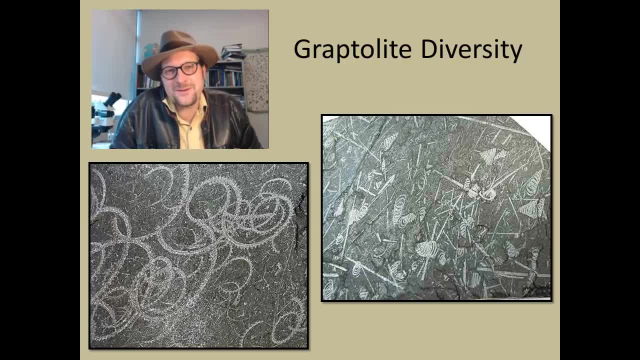 things. They look man-made. Often times you'll see news stories about graptolites as being some sort of gears or some sort of futuristic time machine that's preserved in a fossil record. They're very bizarre. Often times they'll form these spirals that look like gears with the 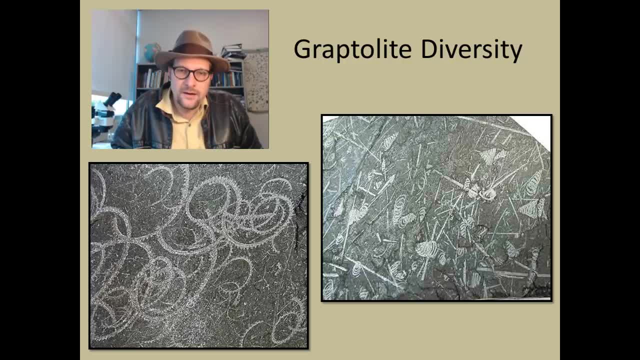 individual apertures that appear almost as if they're like the notches in a gear. Sometimes you see a variety of different forms When these actually were held together. these are actually together as a single unit. they break apart. so some of them have these long, straight pieces. 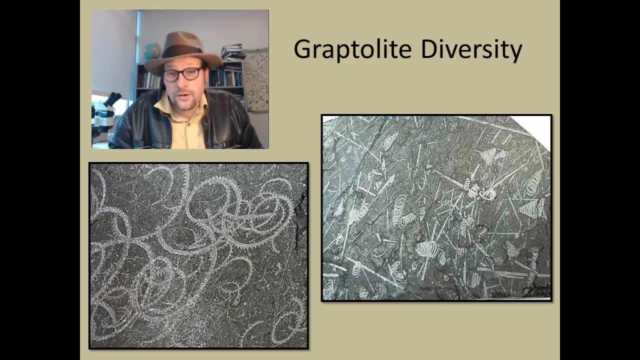 and others, the sort of twisty twirly pieces, most of these really bizarre graptolites or planktonic meaning they floated around and that's how they got out into these black shales that they would fall out, sink down onto the ocean floor and then get buried fairly quickly. so this is my favorite. 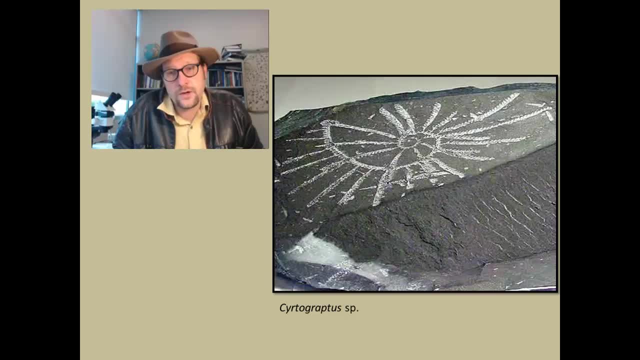 this is kind of the same one that i showed you before, but this is one with those straight edges attached to that spiral. this is crytographius, which is, you know, pretty, pretty amazing little fossil. so these guys have the spirals and then they had the straight edges that came off with. 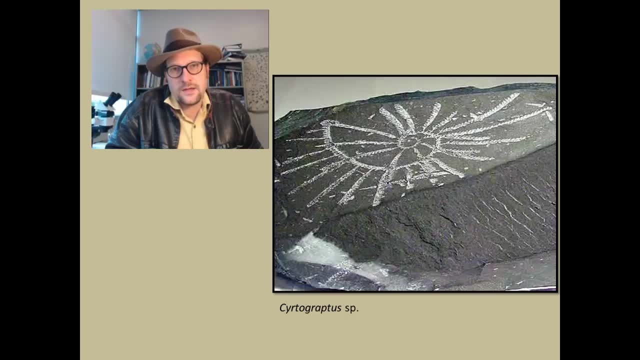 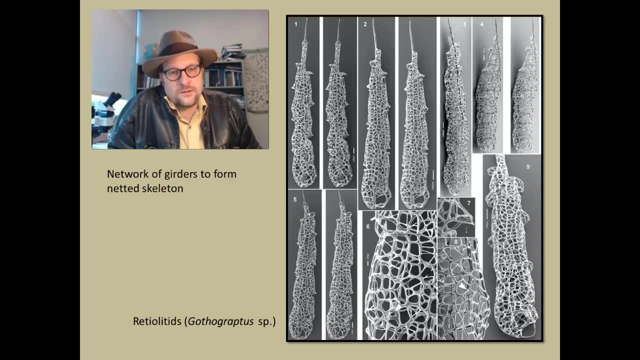 these colonial organisms, and it's thought that they floated planktonically in the ocean waters. some of them are really bizarre. these are the retrolits, this is gothiographus, and they form actually an intricate network of little openings that probably are not that small. so that's one of the things that's really interesting about this one. 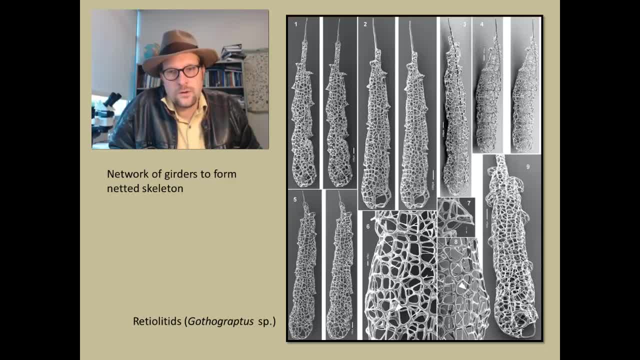 so these guys have the spirals and then they had the straight edges that came off with these colonial organisms. they probably housed individual zooids and was a little colonial uh organism that probably may have been on a stock in a netted skeleton. this is, of course, is collagen. 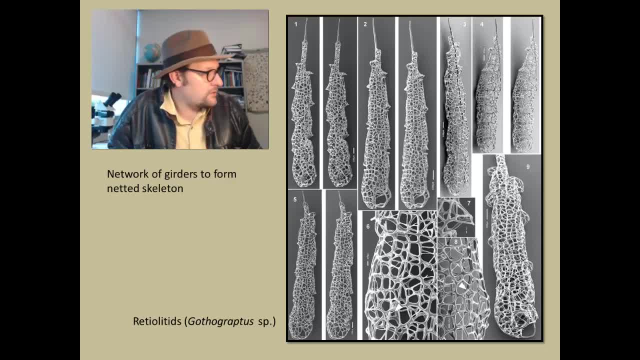 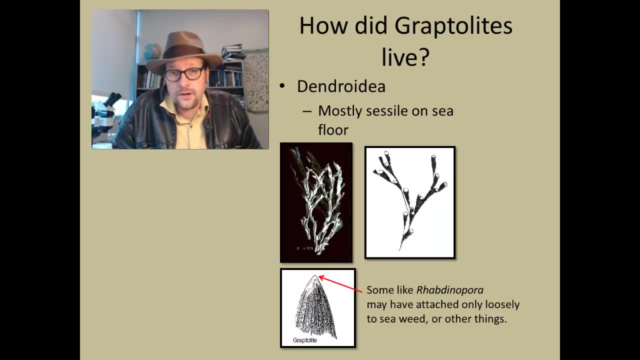 and this is prepared using acid to etch away the rock and leaving behind the organic sort of original skeleton of these organisms- beautiful preservation. most of these are fairly small. they really get over 10 centimeters, all right. so how did graptolites live? well, there's two different. 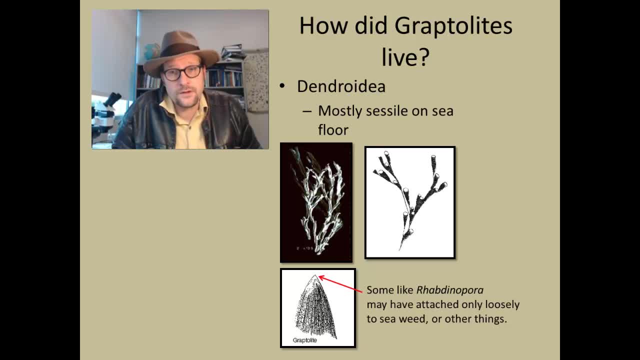 types: the dendroids and the dendroids. the dendroids and the dendroids- the dendroids are the dendroids- were mostly sessile, lived on the ocean floor, branching zooid organisms, again making their skeletons out of collagen rather than calcite, calcium carbonate, like we saw with the bryozoans, but feeding and existing in very similar 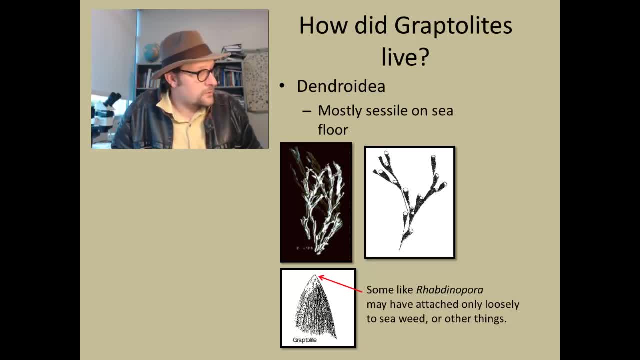 ways as the bryozoans. but these are probably unrelated. they're probably related to the hemi chordates of today. some of them were kind of may have attached loosely to seaweed or something like that and actually formed the dendroids. they're probably related to the hemichordates of today. some of them were kind of may have attached loosely to seaweed or something like that and actually 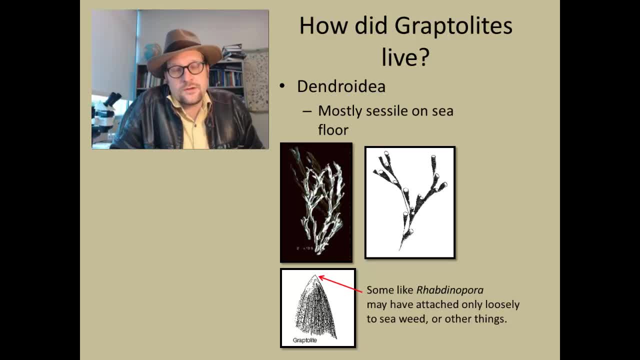 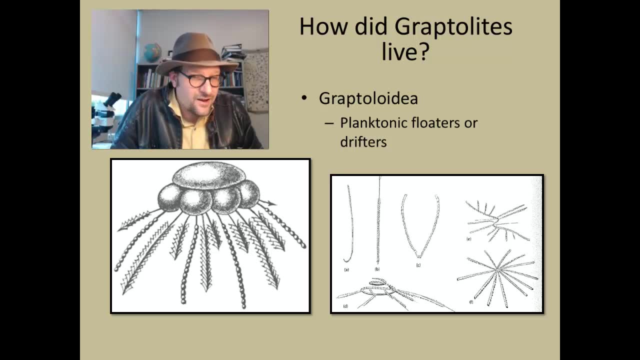 floated upside down, like the graptolite, very interesting groups. the graptoloides- these are the ones that we find in many of the black carbonaceous shales. these are the planktonic floaters, and this is a sort of reconstruction of what one of these might have looked like it's. 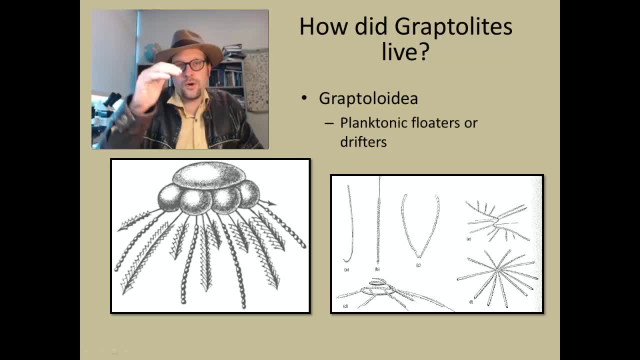 believed that they may have had air sacs to help support them so they would float. so these organisms were maybe colonial, but they actually, with these openings, but probably attached in a network and communicated with each other via a nerve exchange and hence, even though they're colonial, with different types of little zooids that that fed on them, they may have actually been. 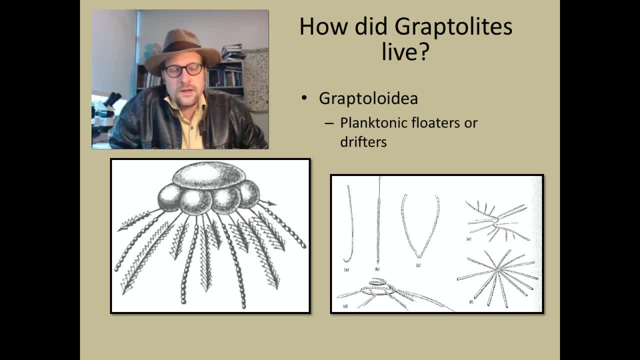 a single organism in terms of their development, to help them float, and so they would float around on the ocean currents, oftentimes in the shallow seas, but then would drift out into deeper ocean waters and filter feed, basically out of the water column. so, because they're filter feeders and 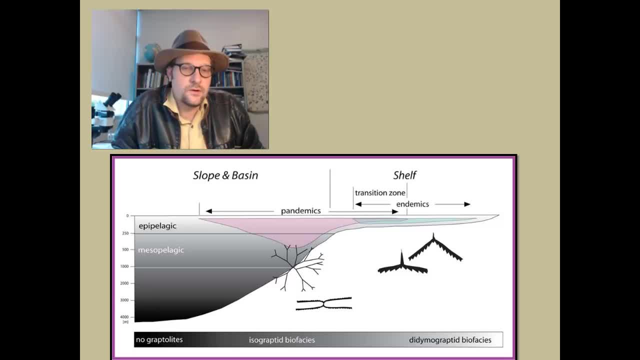 they're also sasa. One of the interesting things that you can get with graptolites is to understand at least how far away you are from the shoreline at particular time periods, how deep the water is. There are groups of graptolites that are called pandemics. that means that they are found. 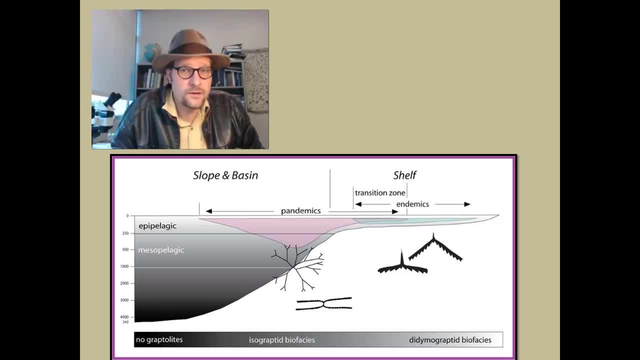 in very wide areas and even out into deeper waters. And then there is the endemics. these are the graptolites that are found in the shallow water systems. many of these are the sessile organisms that live up in the photic zone. 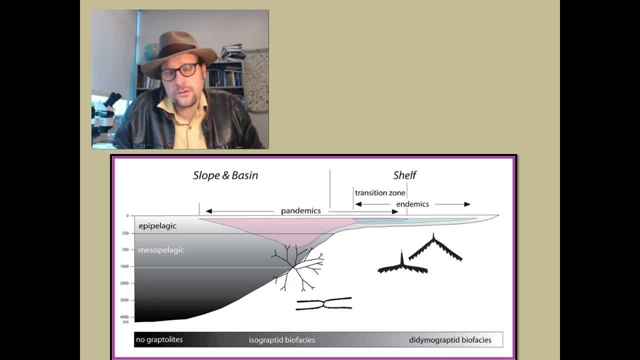 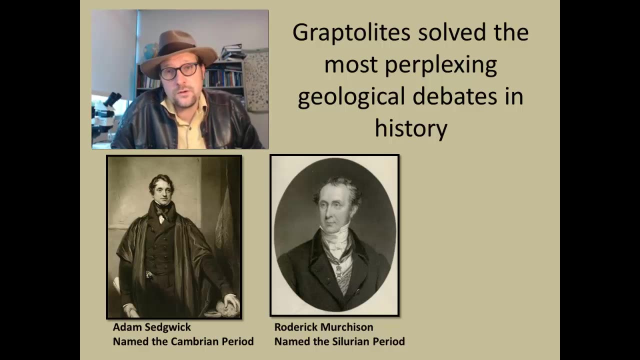 So you can use graptolites to give you an indication of how close you are to the coastline, which is really important if you are doing any sort of basin analysis of the rocks in these marine systems. Now, one of the most interesting stories about graptolites is how they actually came to be. 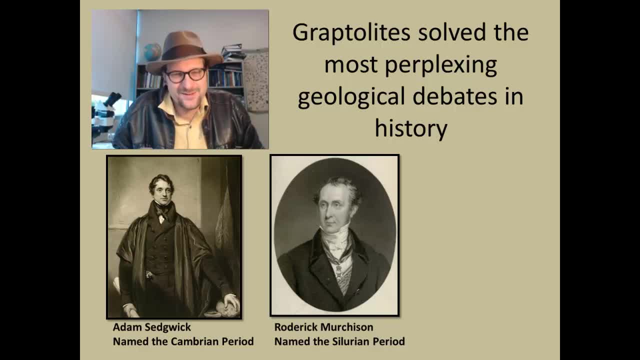 used to solve one of the most perplexing, nasty debates in geological history. I don't know if you know this story, but when geologists were coming up with the geological timescale, there was a lot of debate going on and one of the big debates that was going 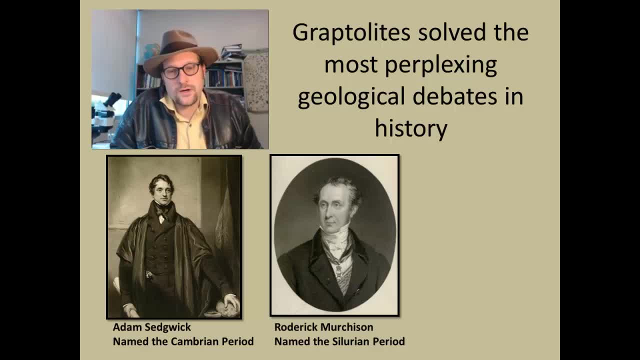 on in Britain was between Adam Sedgwick and Roderick Mutschausen. Now Adam Sedgwick is a big, huge, giant figure because he collected many, many fossils across the British Isles. he is the one that came up with the name Cambrian they came up with 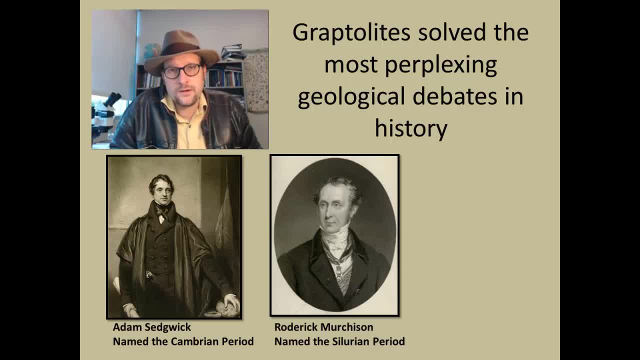 it. Robert Mutschausen is very famous. both he and his wife traveled with Charles Lyell. in fact his wife helped map out many of the rock layers between England and France in the early 1800s. they sort of helped inspire Charles Lyell to write the Principles of Geology. 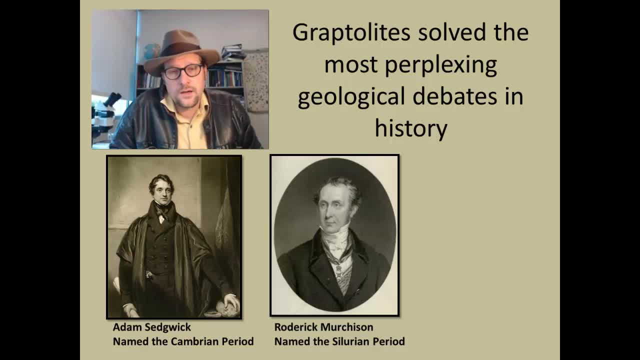 So these guys were collecting fossils. in the 1820s, coming up with these names, Roderick Mutschausen named the Silurian period And they were mapping The parts of Wales and Sedgwick had mapped a bunch of rocks as being his Cambrian age. 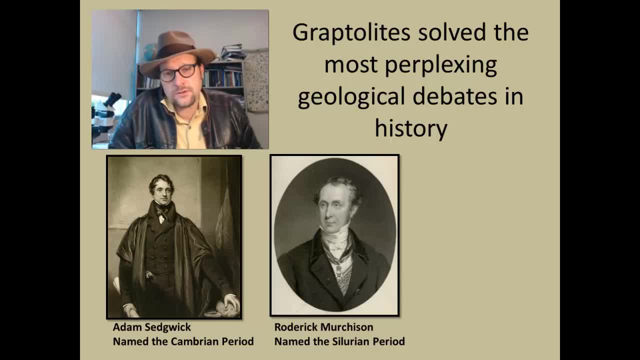 rocks and he was finding fossils there And Mutschausen was mapping on the other side but as he moved in he called that all the Silurian. So you had two camps that developed in England in the early mid 1800s. the camp that belonged 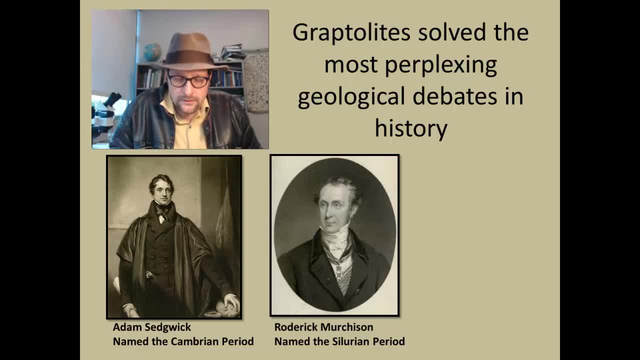 to Roderick Mutschausen believed that all the early time period of these early rocks were Silurian in age and many of the followers of Adam Sedgwick believed they were all Cambrian age And they debated back and forth where they needed to define the line between the Cambrian 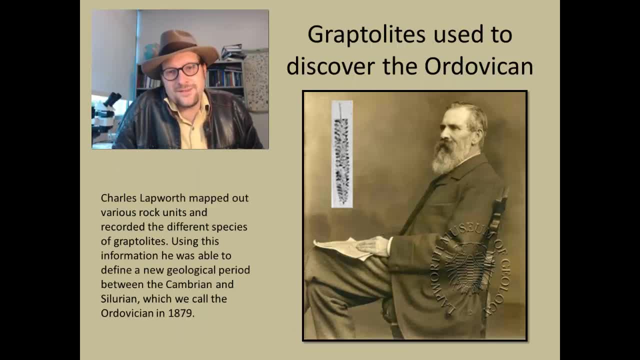 and the Silurian. Well, it wasn't until we get into 1879 that Charles Lapworth began to sort of take on this debate between the Cambrian and Silurian and where to draw that line, And what he ended up doing was that he was finding that many of these rocks were not 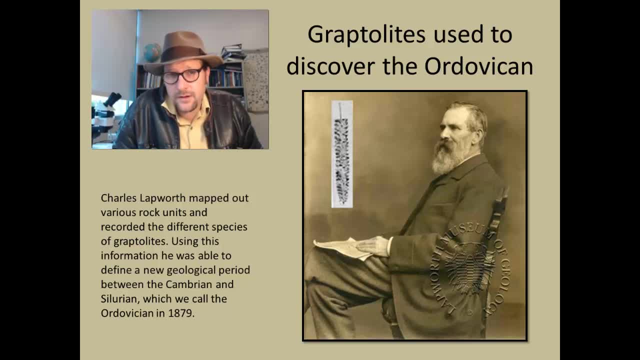 very fossiliferous, except many of them did have graptolites. Now graptolites were sort of ignored by the earlier paleontologists and he realized that these would be very important for defining a period of time between the Cambrian and 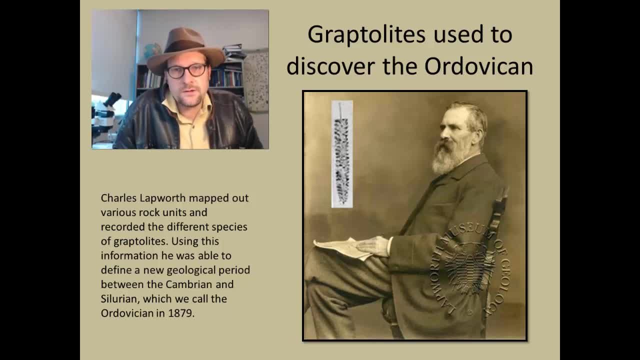 the Silurian, which today we call the Ordovician. So Charles Lapworth was the first to propose a new geological period between the Cambrian and the Silurian, And he defined it based on the appearance of many of these graptolite species that he 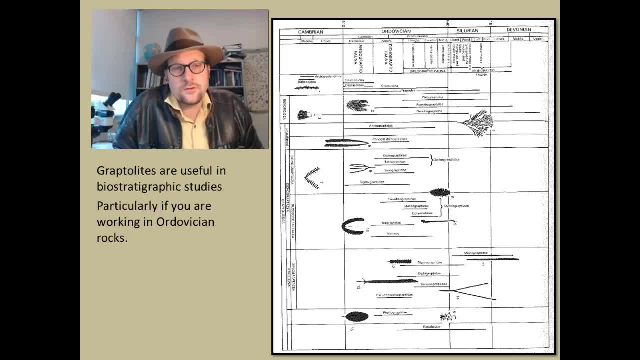 was finding in England. So this is a distribution of graptolites and I mentioned that they are known from the Cambrian to Devonian, And what you'll notice about the Ordovician is that it was a time of great diversity of. 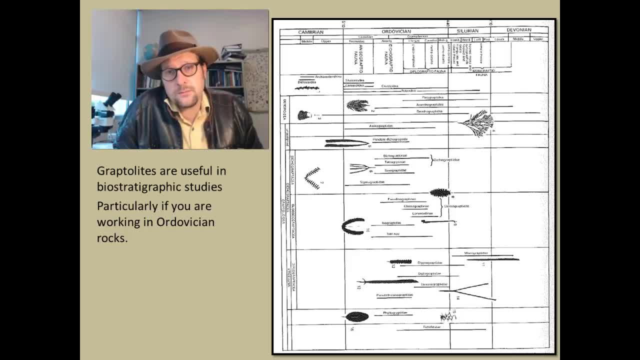 graptolites. So graptolites were particularly well represented in many Ordovician sites, particularly these black shales that had produced many shelled calcium carbonate creatures. So graptolites became a very important biostratigraphic index for rocks in the Ordovician. 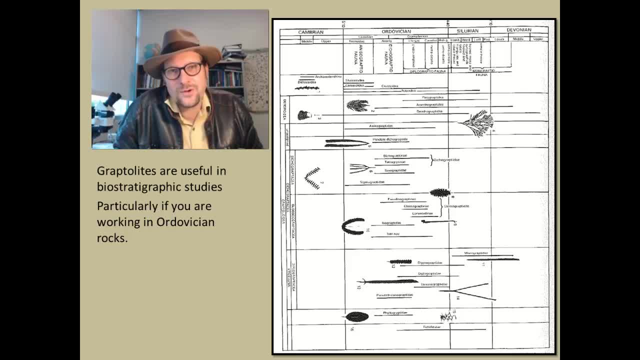 So graptolites of course go extinct at the Devonian. we don't have them living today but they are very important. if you are working in the early Paleozoic Principally you know working that strata between the Cambrian and Silurian, they are very helpful. 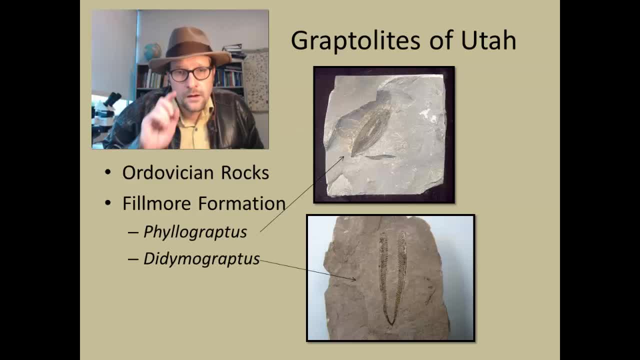 for identifying the difference between the two. Here in Utah we have some Ordovician rocks and I thought I would just highlight two of the common graptolites that define the Ordovician rocks in Utah in the Fillmore Formation. This is Philograftius, which is kind of a leaf shaped graptolite, and the one that is